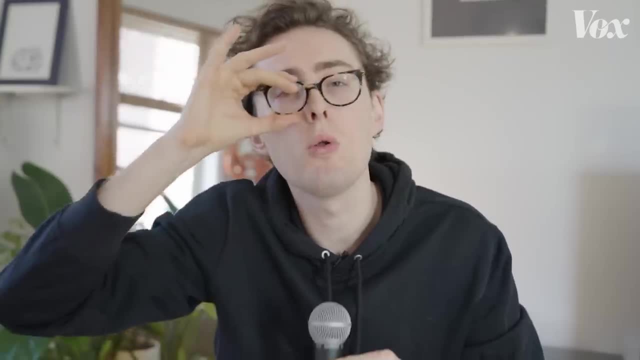 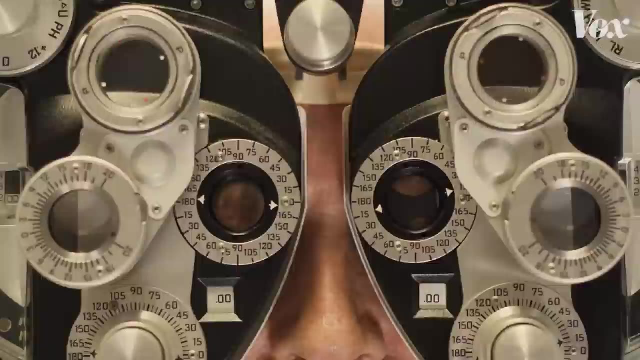 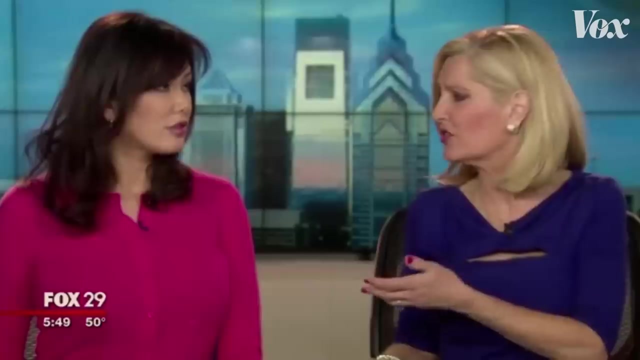 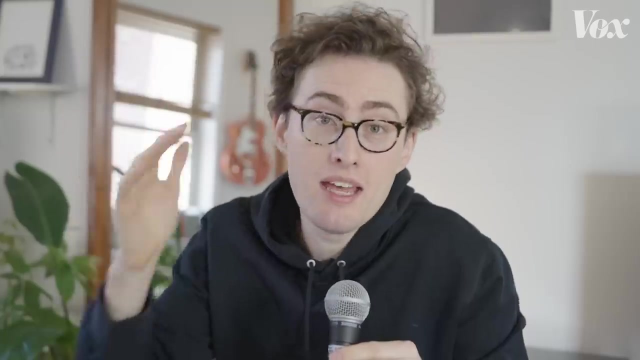 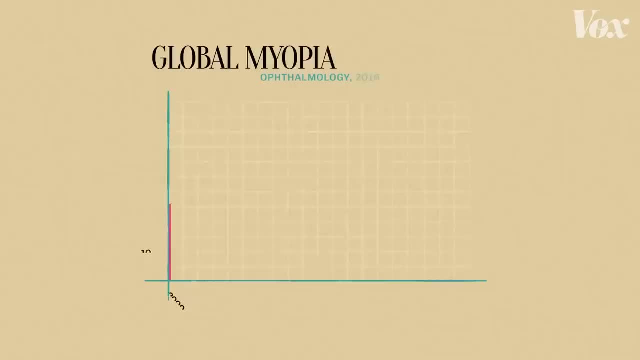 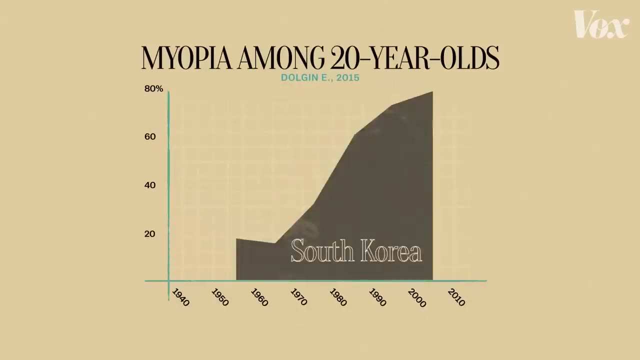 By 2004, that number was up to 42% And if current trends continue, it's estimated that half of the world's population will be myopic by 2050.. In Hong Kong, Singapore, Taiwan and South Korea, rates are already a lot higher than that. 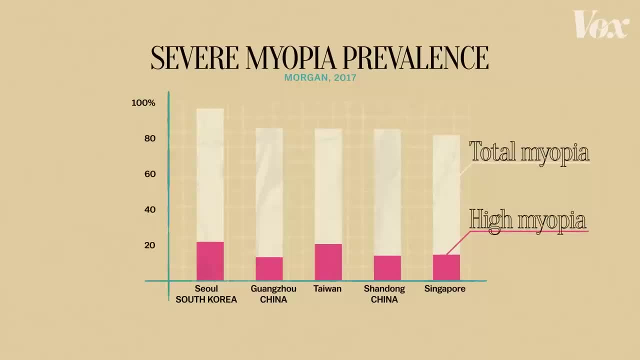 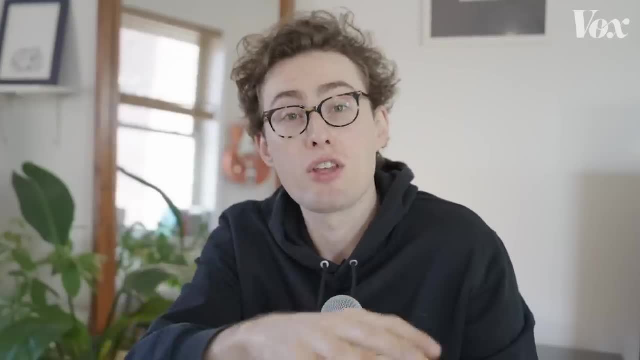 And a growing portion have high myopia, which the WHO categorizes as a prescription stronger than minus 5. That puts them at risk of losing their sight one day. For decades, researchers thought that whether or not you needed glasses was just a matter of genetics, And it partly is Having one. 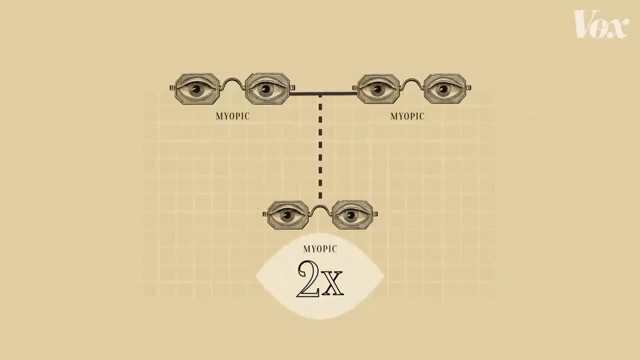 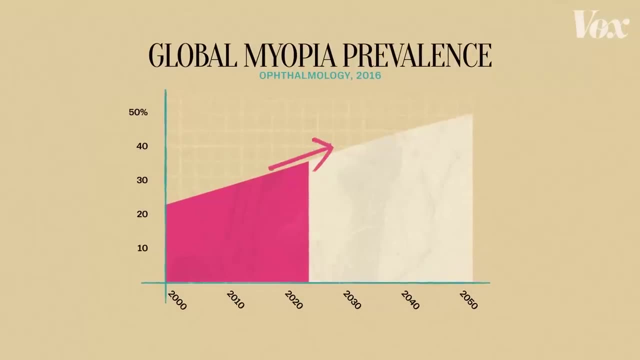 myopic parent doubles your odds of being nearsighted, and having two increases the odds five-fold. But human genetics don't change this fast. The abruptness of this increase suggests that this change is environmental. Something about the way we live today is making it harder. 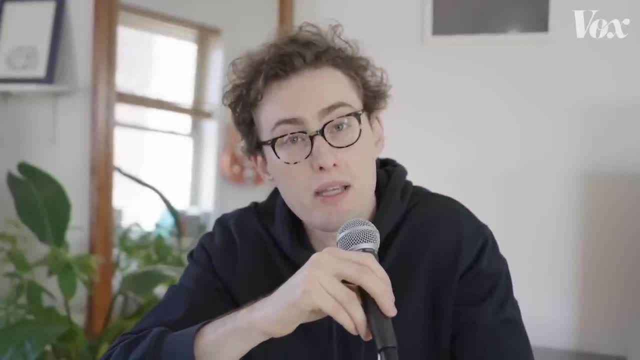 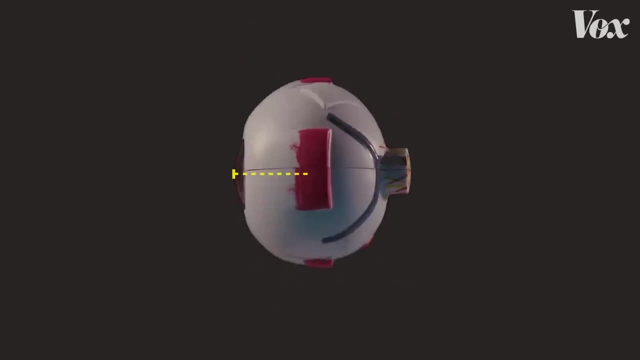 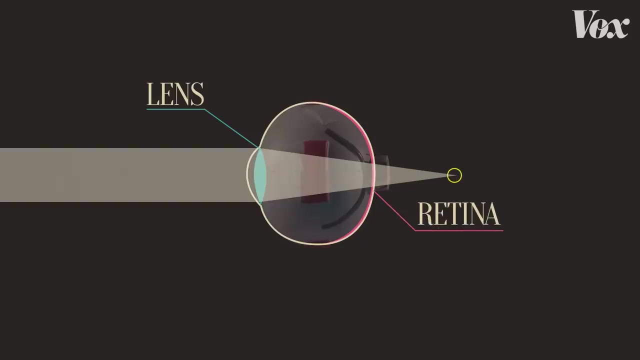 and harder for people to see at a distance. So what could it be? Most people are born with eyes that are too short from front to back. In this shape, the lens focuses images behind them, the retina, that's the light-sensitive tissue at the back of the eye. 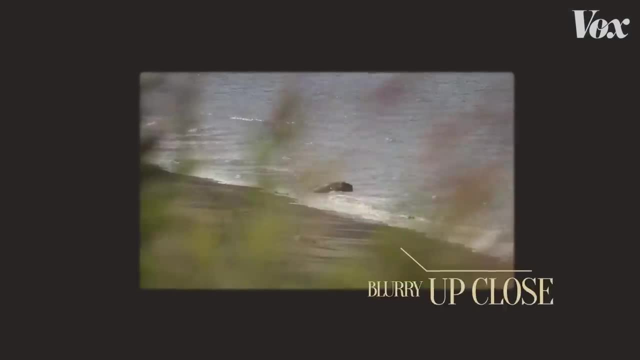 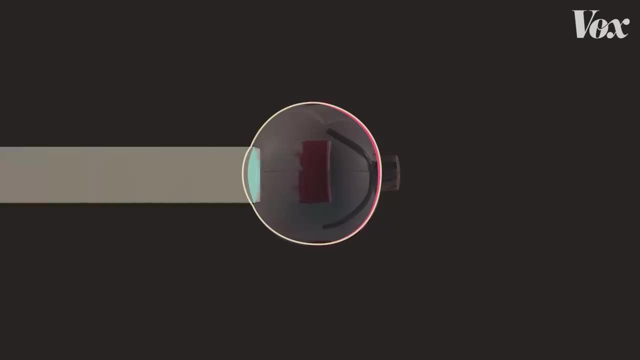 That makes the eye hyperopic or farsighted: blurry, up, close and clear from far away. But as we grow up, our eyes grow too, until they reach a spherical shape. In this shape, the lens focuses light directly onto the retina and produces a clear image. 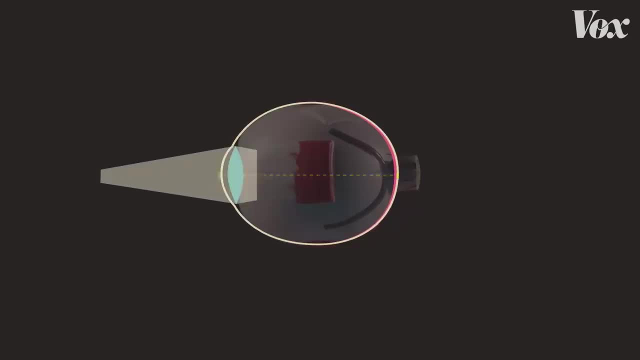 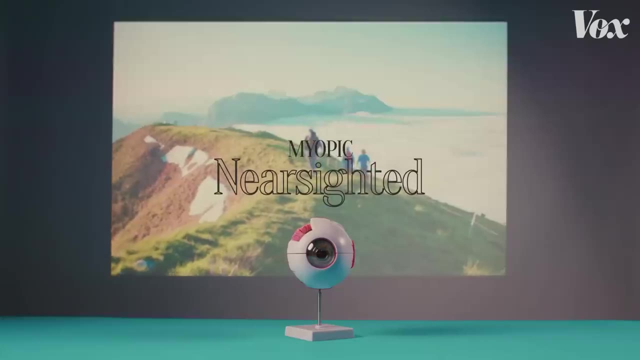 But sometimes the eye keeps growing longer. In this shape, the lens can focus up-close images onto the retina, but at a distance, images focus at a point in front of the retina, making distance vision blurry. So all of us with myopic vision, we can see the retina, but we can't see the retina. 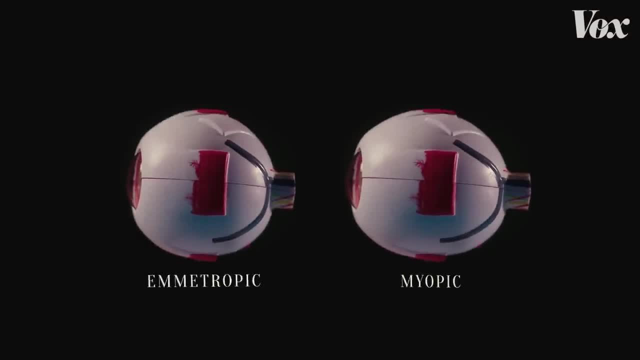 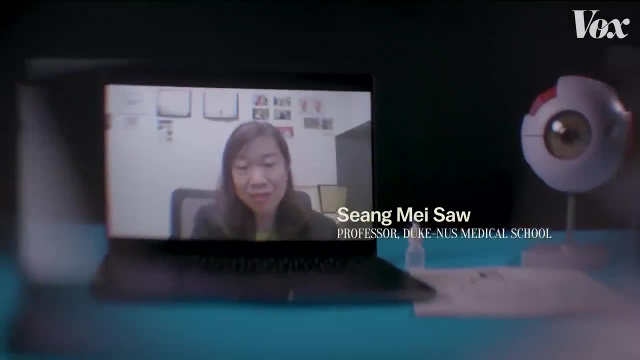 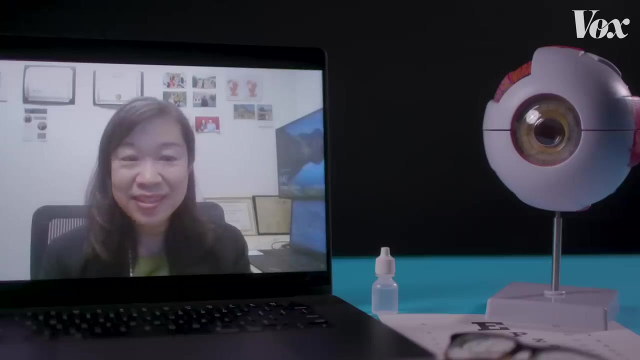 Myopia just have eyeballs that have grown too long. The eye does not look like a basketball anymore, It looks more like a rugby ball. That's Xiangmei Sa. She's a myopia epidemiologist and physician in Singapore. It is a lifelong disease, So once you're myopic, it doesn't regress. So what's making more and more people's eyes grow longer than they should? The evidence points to the way we spend time in childhood and adolescence. That's when our eyes grow fastest. So it's when most people's myopia develops and then stabilizes, though it can develop later if you abuse your vision enough. 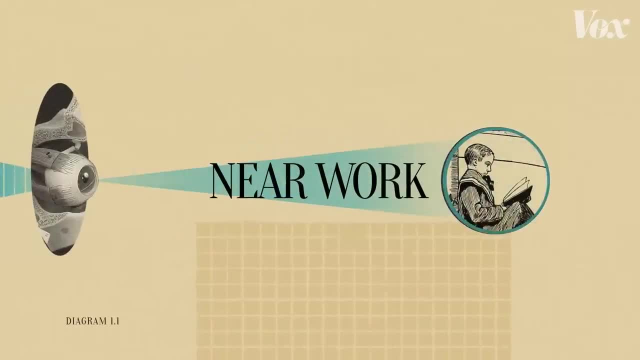 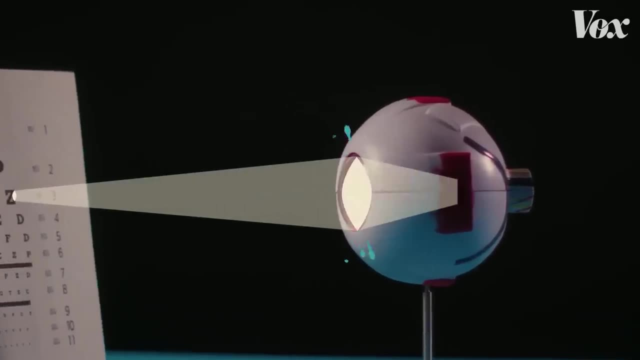 Two factors in particular have the biggest influence: Near work, or the time that we spend looking at things up close, and how much time we spend indoors. In a healthy eye, muscles have to squeeze the lens in order to focus up-close images onto the retina. 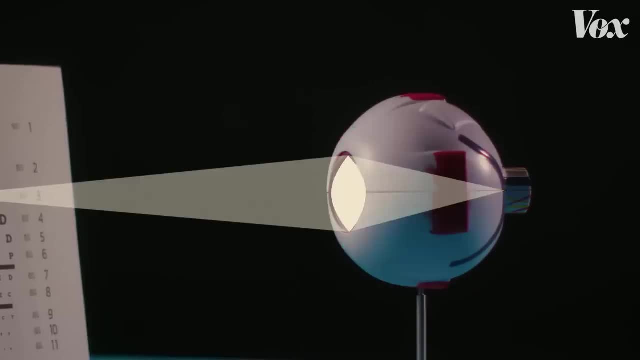 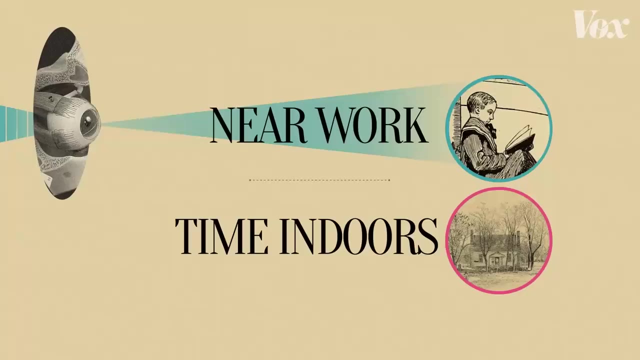 So some experts theorize that if your eyes grow up straining to look at things up close a lot of the time, they'll just grow longer to reduce that strain. But the evidence on this explanation is mixed. The stronger explanation is time spent indoors. 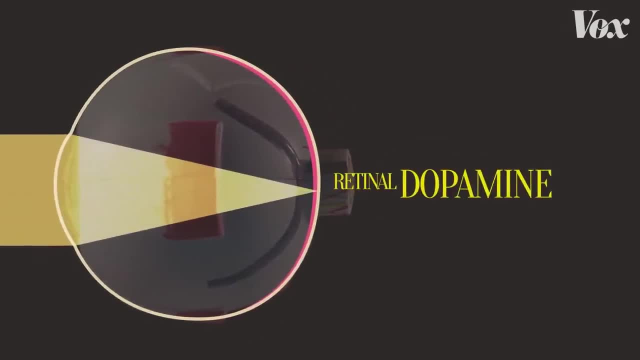 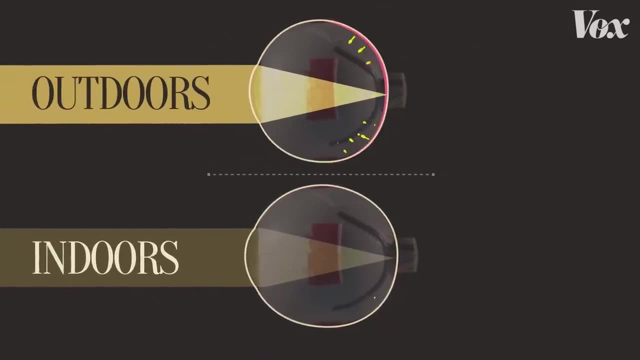 Exposure to bright outdoor light stimulates the production of dopamine in the retina. This neurotransmitter regulates the eye's growth. Without enough dopamine, the eye doesn't know when to stop growing, And indoors it's hard to get enough. The light from the sun has up to 100,000 lux on a sunny day. 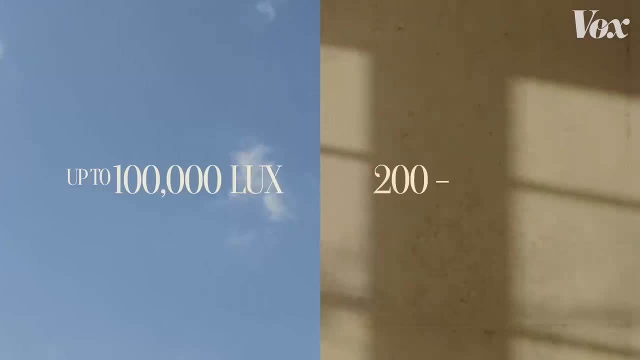 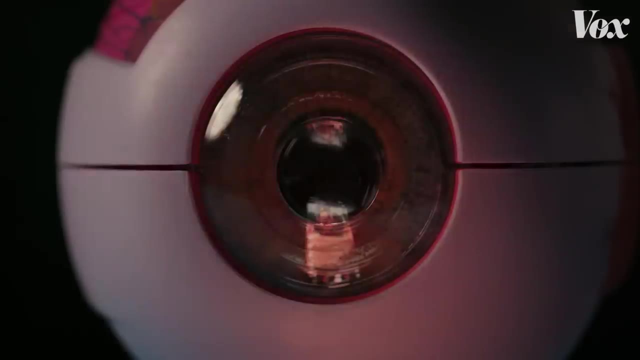 whereas in a room the light levels generally are only about 200 to 300 lux. But between electronic devices and early emphasis on academics, eye experts believe that children today are growing up with a combination of too little daylight and too much time doing things up close. 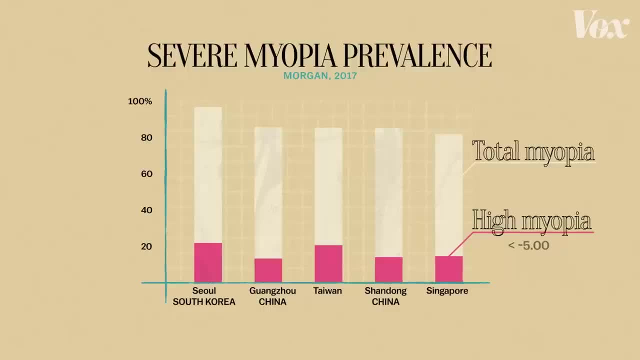 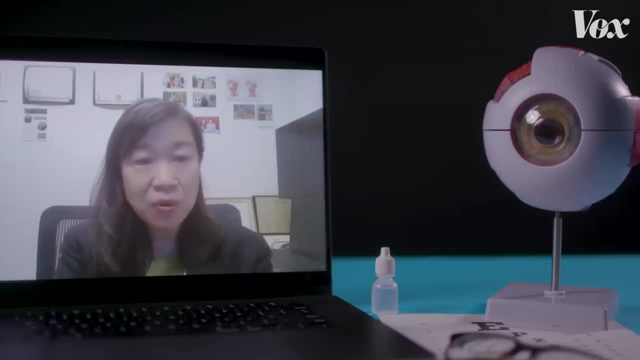 And nowhere is that more apparent than in East and Southeast Asia. Children in Asia are not spending that amount of time outside. This could possibly be because of the education system has become much more competitive. The children have a lot more homework, They attend tuition centers and they spend more time reading and writing. 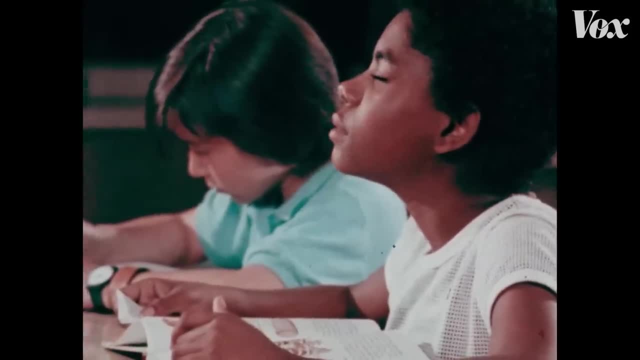 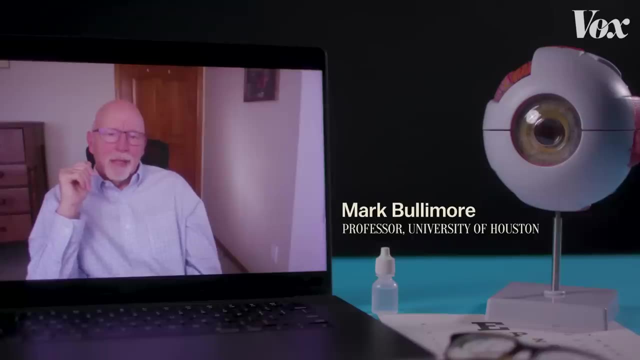 Kneading glasses or contacts to see for the rest of your life is obviously inconvenient, But in the long term the consequences of that distorted eyeball shape can become serious. University of Houston professor of optometry, Mark Boulamore, explained this to me. 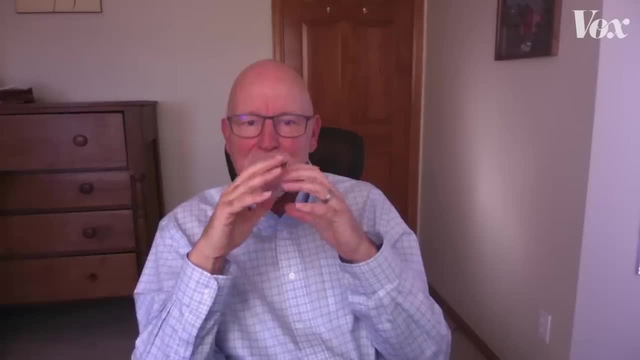 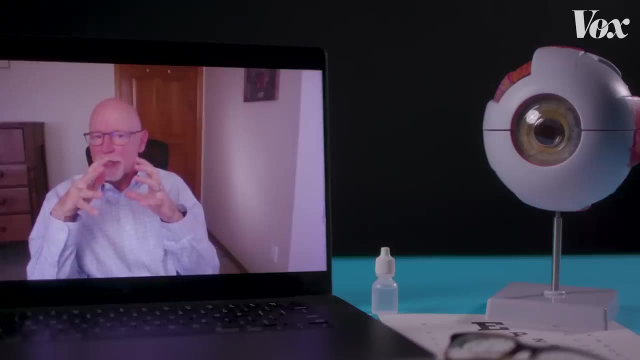 Mark Boulamore, University of Houston, professor of optometry. University of Houston. professor of optometry. You're born with a finite amount of tissue that make up the various coats of your eyeball. Excessive elongation of that quite simply places additional stress on those structures. 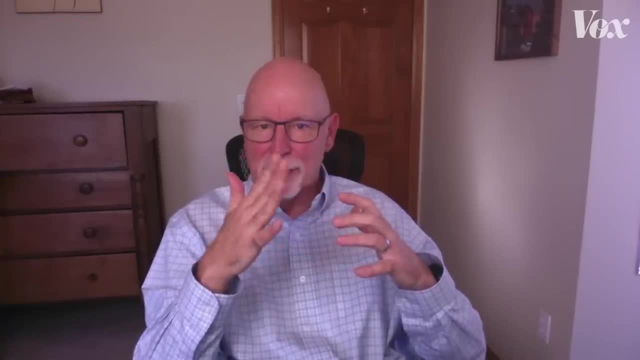 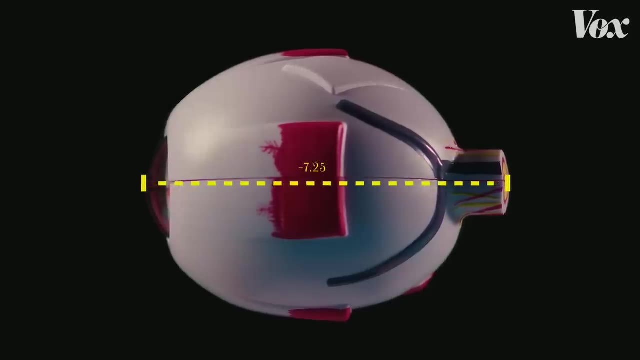 The retina has been stretched so much that it starts to break and then sort of peel off like an old piece of paint. The longer those eye structures are stretched, the higher the risk of disorders like myopic macular degeneration, retinal detachment.